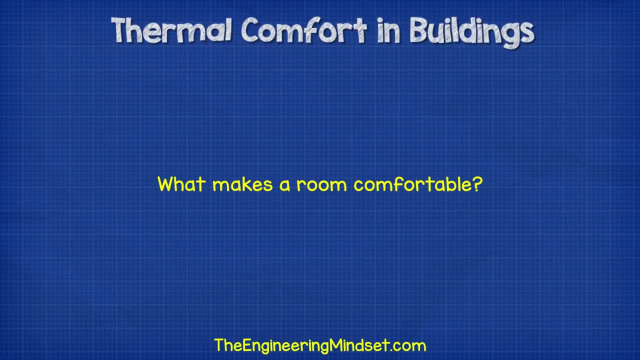 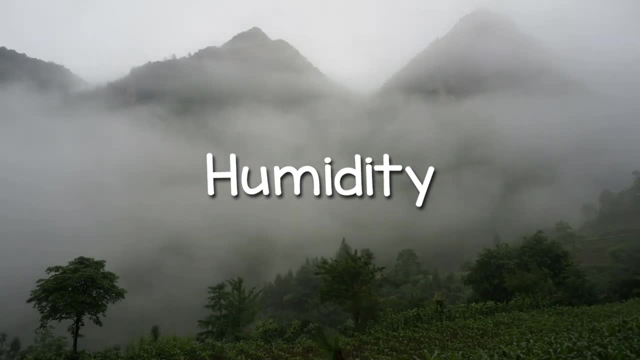 we can improve bad ones. When we consider what makes a room comfortable, we tend to think of temperature first. That's true, but there are other things we need to consider also, like the humidity, the air velocity, the radiant temperature, the metabolic rate. 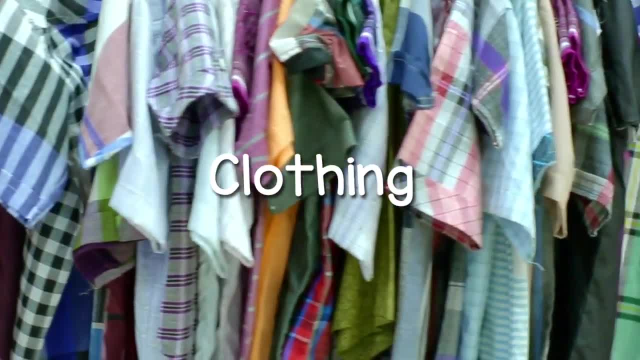 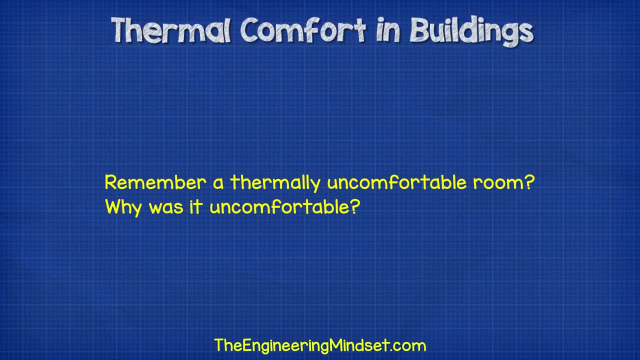 and also our clothes. We'll go through each of these a little later in the video and discuss how they impact our built environment. But if we think about times when we've been in a room which was firmly uncomfortable, then the air was probably too hot or cold, the humidity way too high and 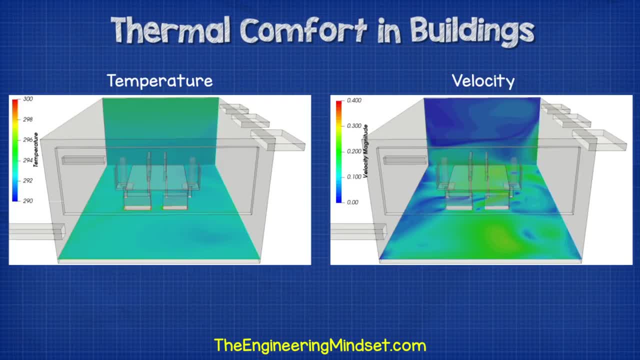 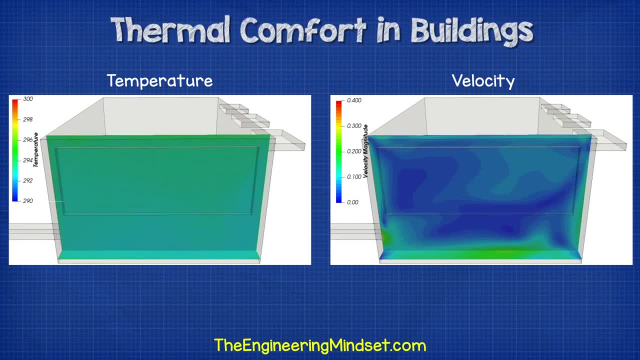 the air circulation was either not enough or far too much. We can simulate and even compare the performance of different designs quickly and easily using CFD or Computational Fluid Dynamics. These simulations on screen were produced using a revolutionary cloud-based CFD and FEA engineering platform. 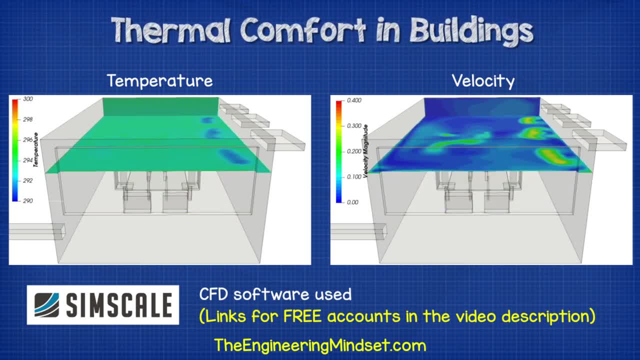 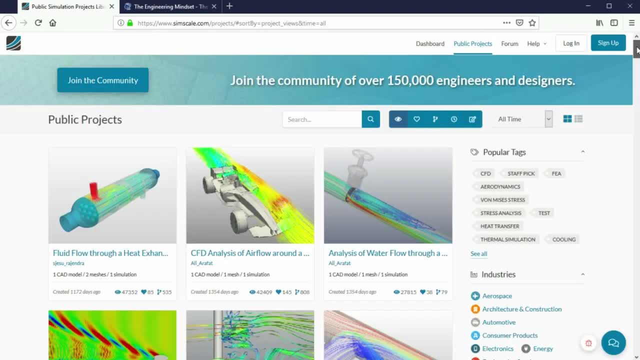 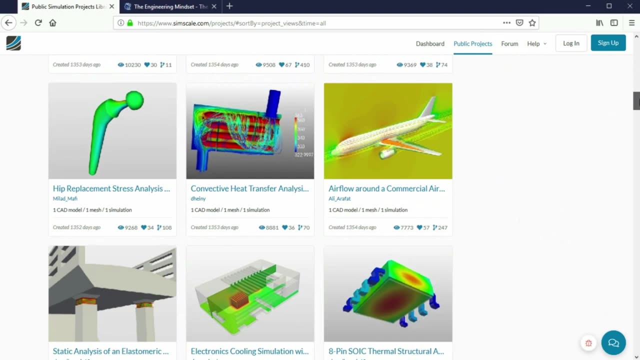 You can access this software using the links in the video description below, and they offer a number of different account types, depending on your simulation needs. SimScale isn't just limited to thermal design. it's also used for data centres, AEC applications, electronics design, as well as structural analysis. Just a quick look through their site and you. 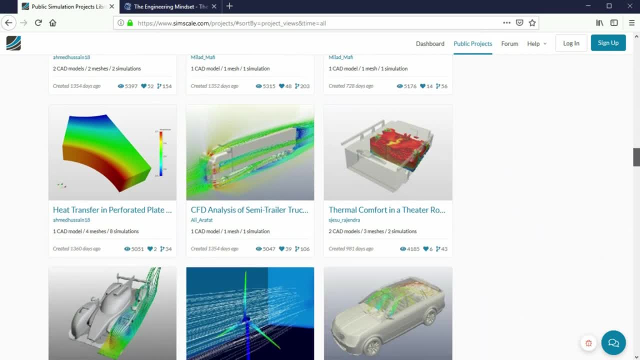 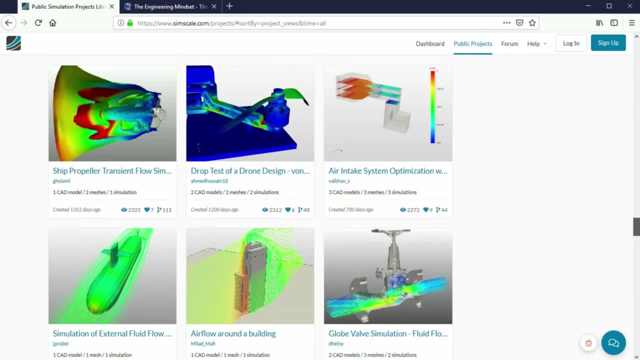 can find thousands of simulations for everything from buildings, HVAC systems, heat exchangers, pumps and valves to race cars and aeroplanes, which can all be copied and used as templates for your own design. Thanks for watching. If you're interested in learning more about CFD and CFD analysis, they also offer free 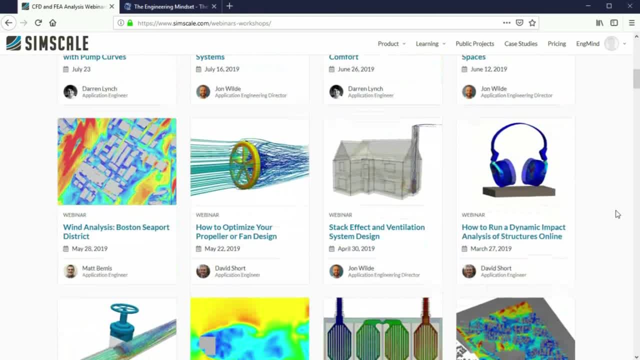 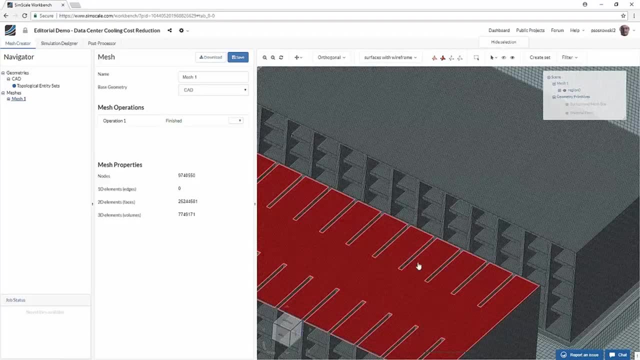 webinars, courses and tutorials to help you set up and run your own simulations. If, like me, you have some experience creating CFD simulations, then you'll know that this type of software is usually very expensive and you would need a very powerful computer to. 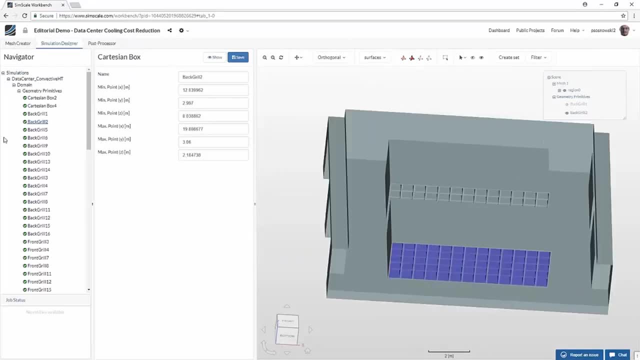 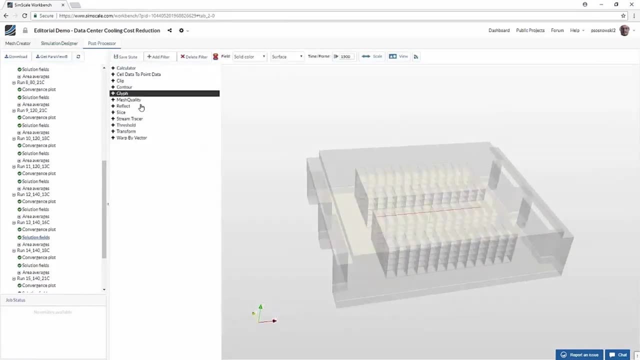 run it. However, with SimScale, it can all be done with a web browser. As the platform is cloud-based, their servers do all the work and we can access our design simulations from anywhere, which makes our lives as engineers a lot easier. So, if you're an engineer, a 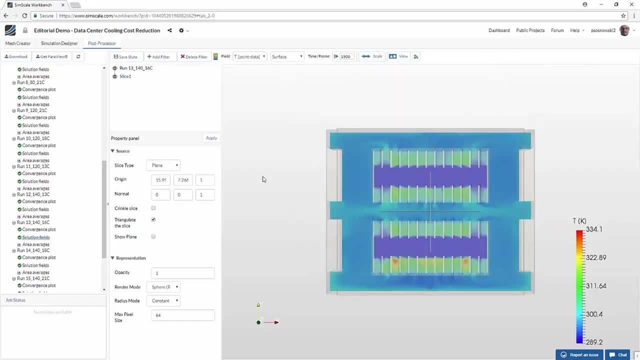 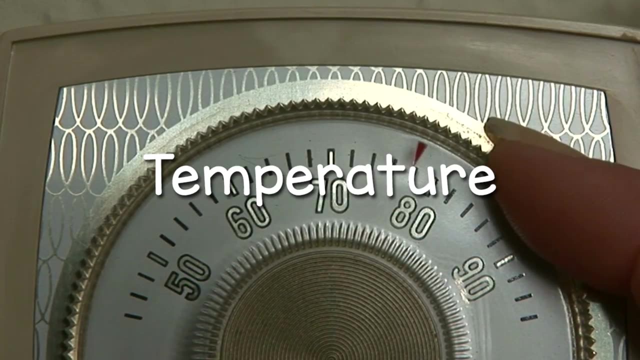 designer, an architect or just someone interested in trying out simulation technology, then I highly recommend you check out this software and get your free account by following the links in the video description below. Temperature: The temperature of a room is one of the most noticeable factors in comfort Our bodies 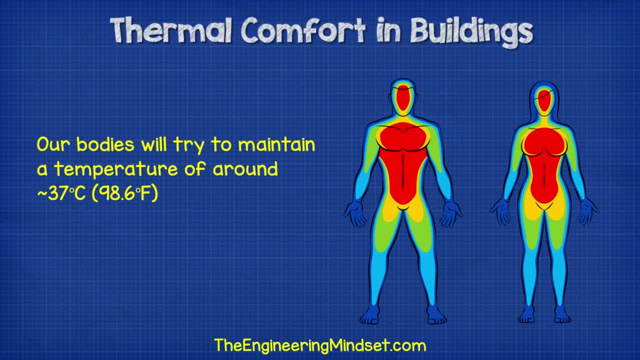 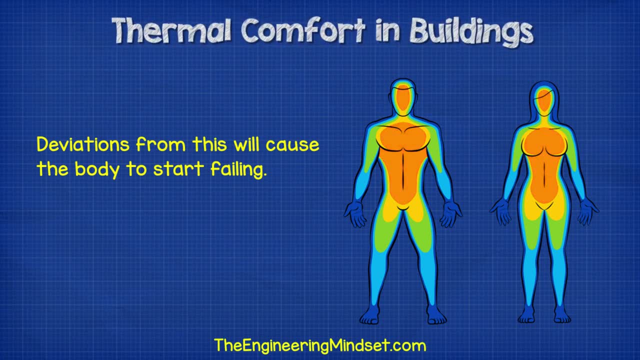 will try to maintain a temperature of around 37 degrees Celsius. This is to keep our internal organs functioning optimally. If our core body temperature deviates from this by just a few degrees, our bodies will begin to fail. We can lose confidence. we can lose confidence. we can lose confidence. 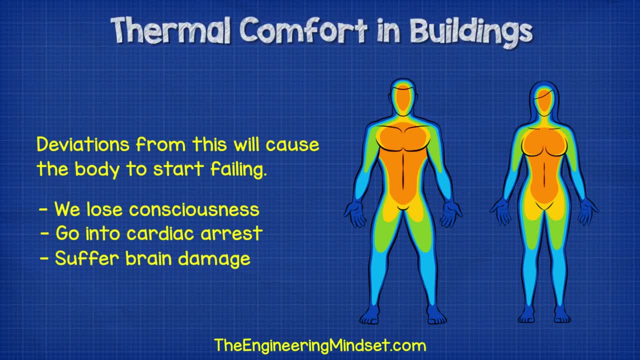 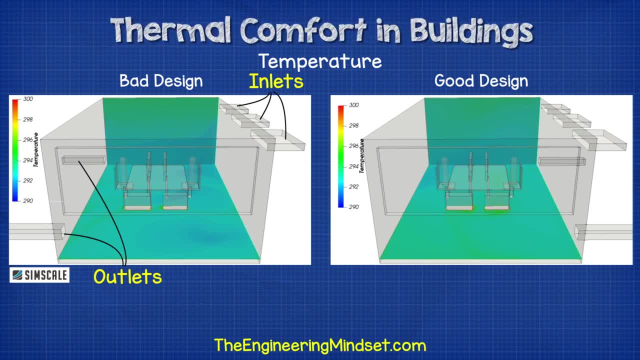 design has 3 inlets at the top right with two outlets at the bottom left. The occupants are sitting at desk in the centre of the room, represented by the cilinders. As we look at the temperature of the air, we can see that the cold air is pouring out. 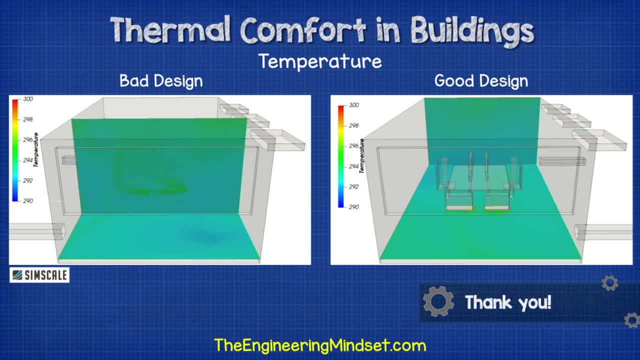 of the inlets and the central grille is discharging directly onto an occupant, So this is clearly a bad design. The purpose here is not to make them getjęstήσще. they don't have enough energy that they can manage, and all they want to do is create a completely different layout. 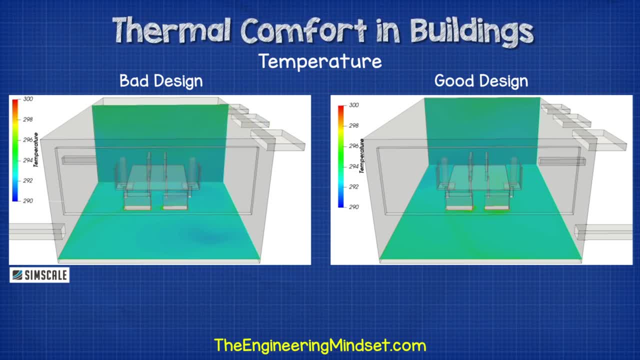 The person on the left might be quite comfortable, but the person under the discharge is going to feel very cold and will probably become unwell. Now, in the improved design, the outlets have been moved under the inlets and only the central duct is being used to deliver the same quantity of air. 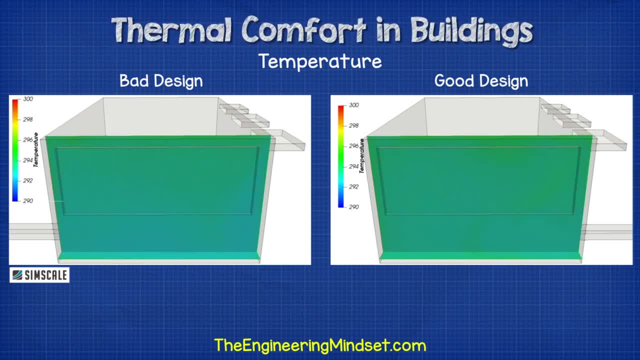 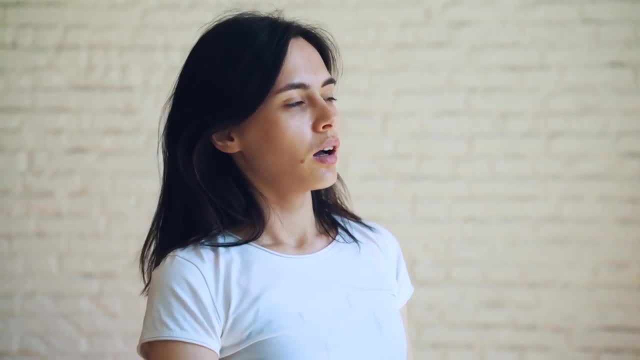 However, now we see that the distribution is spread across the upper regions of the room, giving a more stable and equal environment. Both occupants now experience the same conditions. When we are too hot, our bodies will sweat. This liquid will form a thin layer over our skin, which will evaporate. 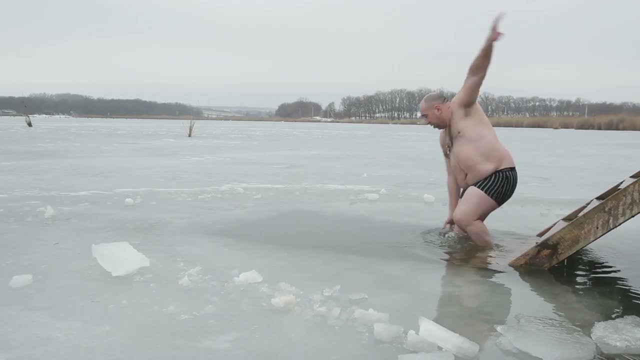 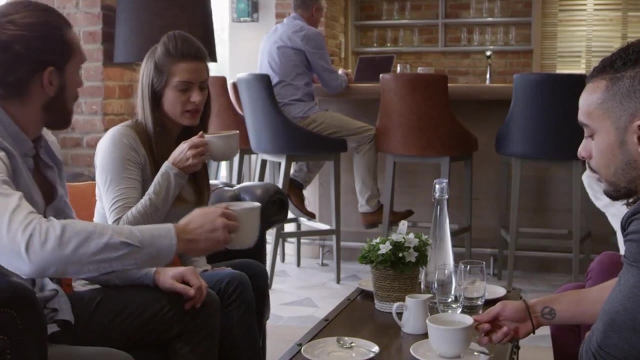 As it evaporates, it will carry the heat away and cool us down. When we get too cold, our bodies will shiver. This causes rapid movement of the muscles, which will generate heat to warm us up. So we need to be in a room which is not too hot and not too cold. 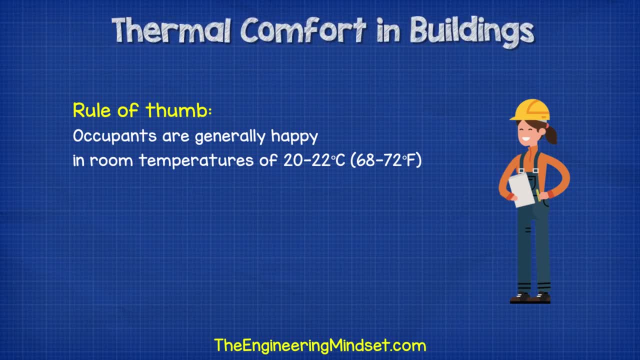 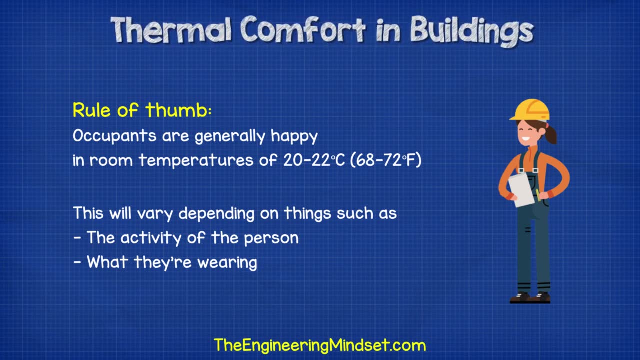 As a rule of thumb, occupants will feel comfortable when the room temperature is around 20 to 22 degrees Celsius, but this will vary depending on things such as the activity of the person and also what they are wearing. To give you an example of a real world design, this is an extract from a SIBSE TM31 building. 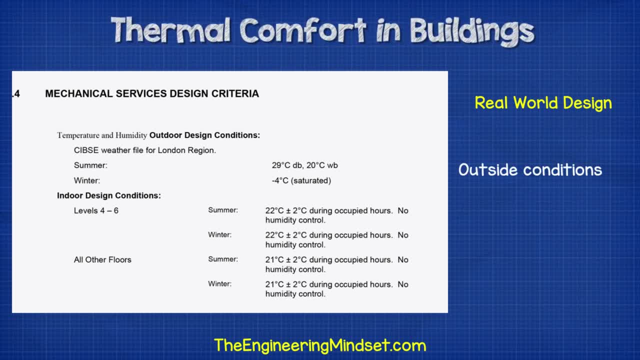 logbook for a new office building in London. You can see the building was designed for outside conditions in the summer of 29 degrees Celsius and in the winter it's negative 4 degrees Celsius. The office area within the building is designed to be 22 degrees Celsius, with a 2 degree buffer. 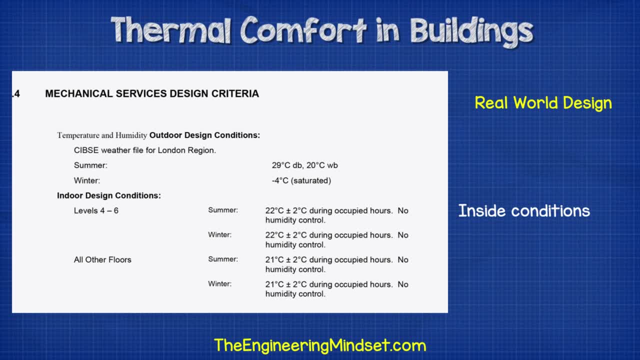 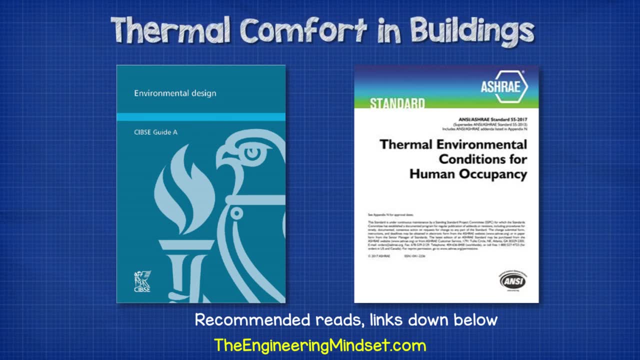 That means it can be anywhere from 20 to 24 degrees Celsius. You can also see that this one has no humidity control, but we'll look at that a bit later. This is an example of a real world design. If you want to get deep into the details of design, then ASHRAE 55 and SIBSE Guide A. 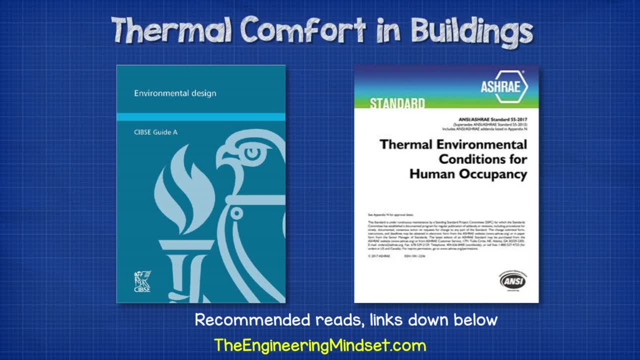 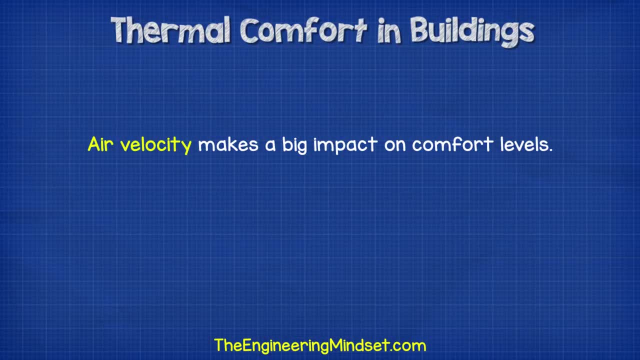 are some of the most widely used industry guides for thermal design and comfort. I'll leave some links in the video description if you want to check those out. Air Velocity: Air velocity is another aspect which will make a big impact on a person's comfort levels. 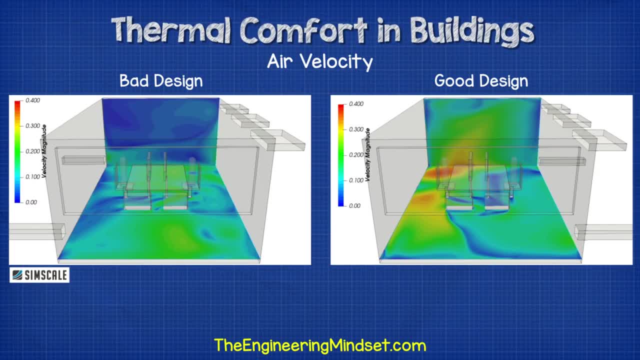 The faster the air moves, the greater the heat exchange will be. So, as we see in the BAD design, the person on the right won't be comfortable because the air is moving fast over them, and so the heat is going to be leaving them uncomfortable. 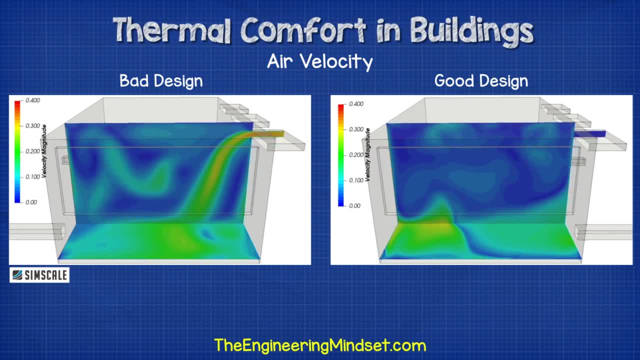 So the person on the right won't be comfortable because the air is moving fast over them, and so the air is moving fast over them, and so the air is moving fast over them, and so the body is moving very rapidly. In the improved design we have a higher velocity over the occupants, but this time it isn't. 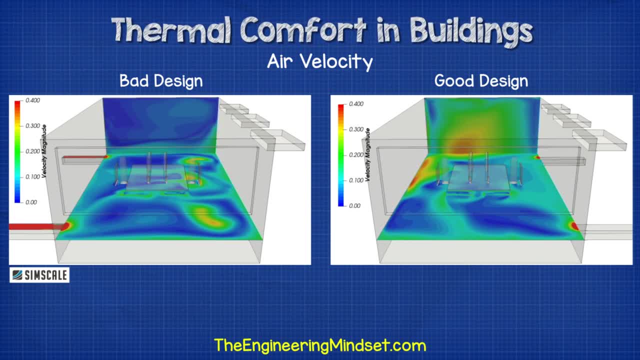 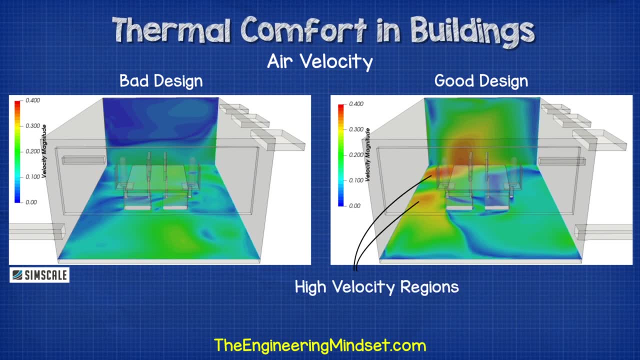 falling directly on them. The occupant on the left might just feel this on the top of their head, and probably so if they were to stand up. The occupant on the right is not falling directly on them. There's also a high velocity region under the ankles, so some improvements could still. 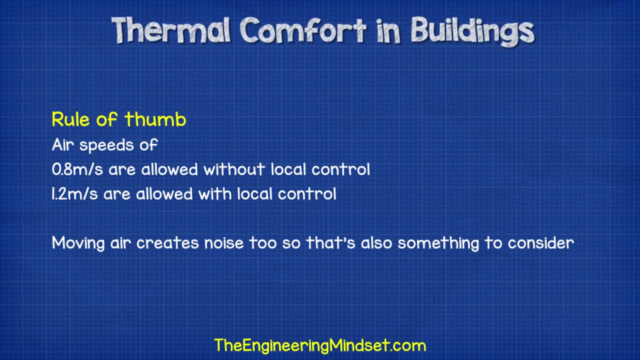 be made for the location and quantity of the grills. As a rule of thumb, airspeeds of up to 0.8 ms are allowed without local control and 1.2 ms with local control. Air is faster in the BAD design, so it's not a problem. 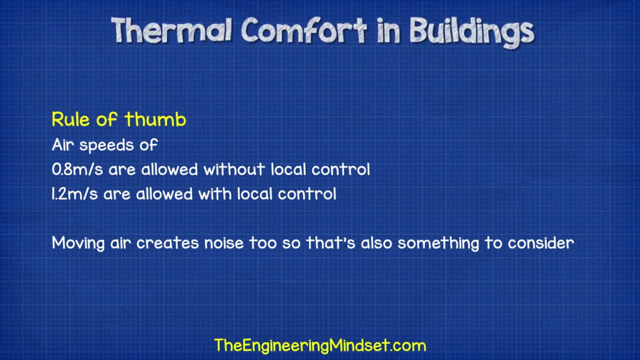 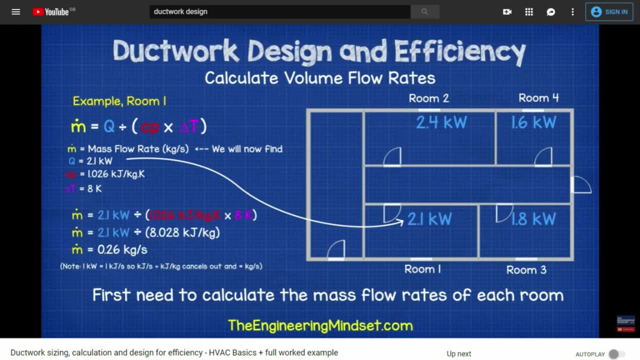 noise too, so that's also something to consider. There are design limitations for ductwork velocity, and we've covered this in our previous video, where we designed a simple duct system. Do check that out for more details. Humidity: When we talk about humidity, we're talking 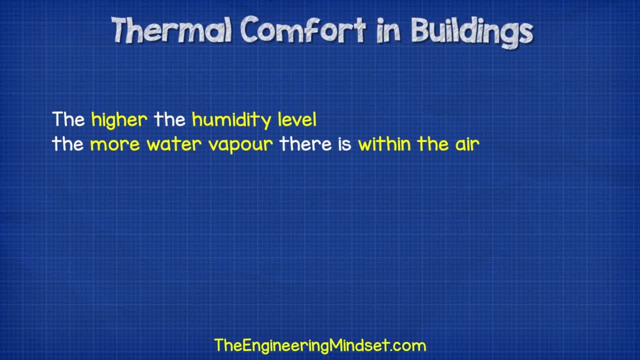 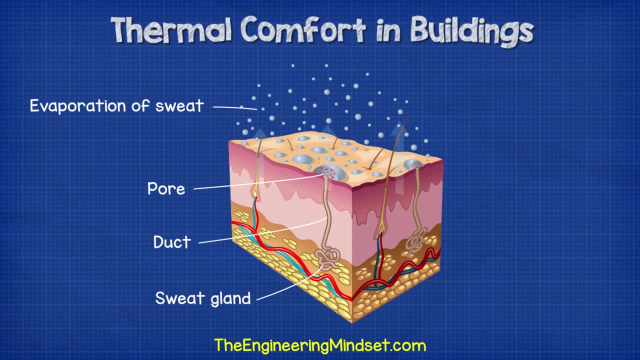 about the amount of moisture in the air. The higher the humidity level, the more water vapour there is within the air and that will make it harder for our bodies to reject its unwanted heat. That's because our bodies sweat to evaporate the heat away. but if there's 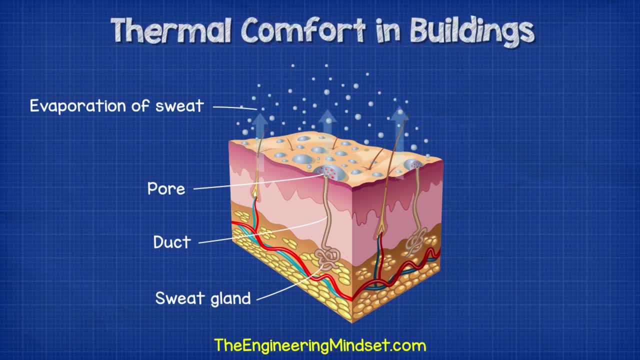 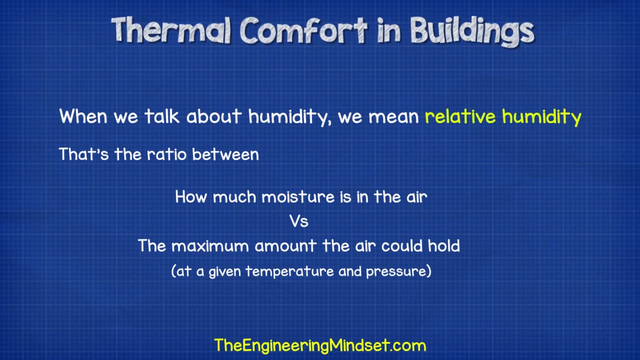 too much moisture in the air, then the sweat can't easily evaporate and we will overheat. When we talk about humidity, we mean relative humidity, which is the ratio between how much moisture is in the air versus the maximum amount that the air could hold at a given. 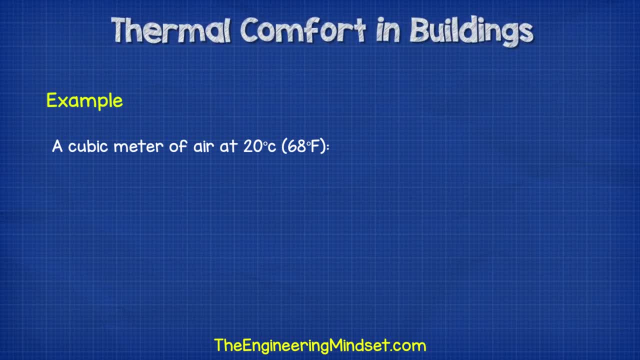 temperature and pressure. For example, a cubic metre of air at 20°C or 68°F with 50% relative humidity will contain around 8g of water, but at 100% humidity this air will hold 17g of water. 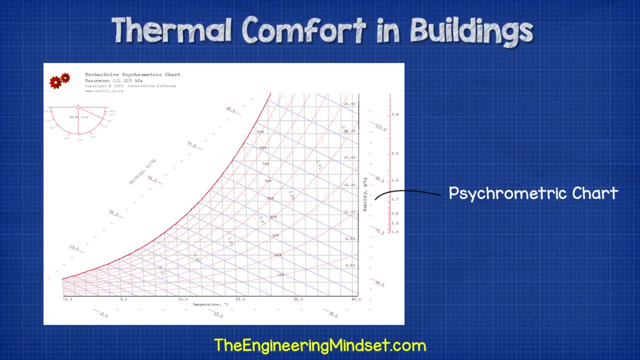 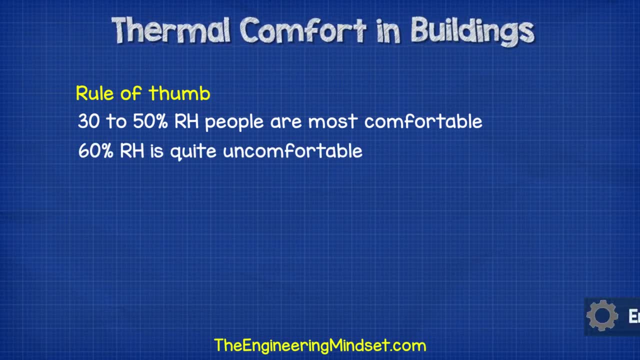 We can read this information in the description below. As a rule of thumb, people are comfortable in 30-50% relative humidity. 60% is quite uncomfortable, and as we reach 70% relative humidity or above, that's when we start. 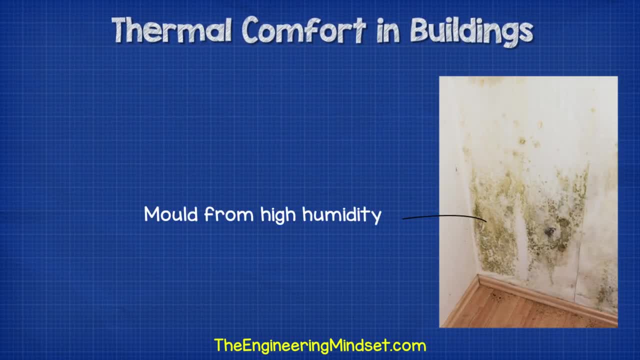 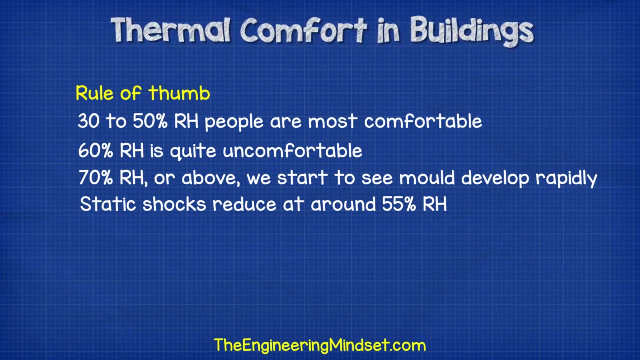 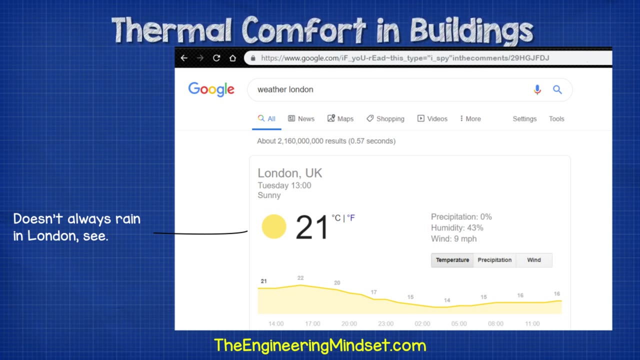 to see mould developing rapidly. You'll probably notice this in bathrooms, where there's high moisture levels and very low ventilation. We can also reduce static shock by keeping our environment at around 55%. As an example, if I google the current weather for my location, we can see that it's showing 21°C outside and 43% humidity, and that's 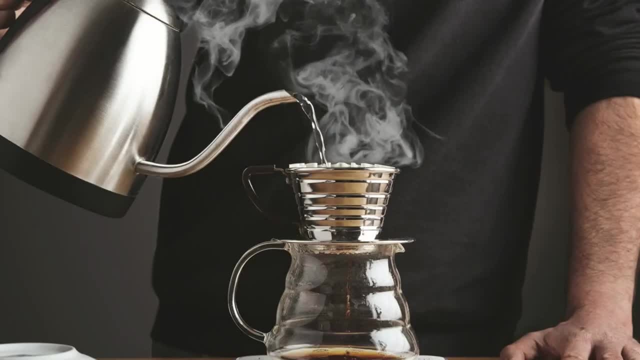 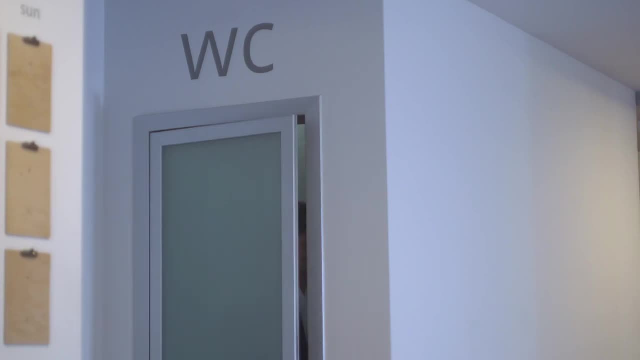 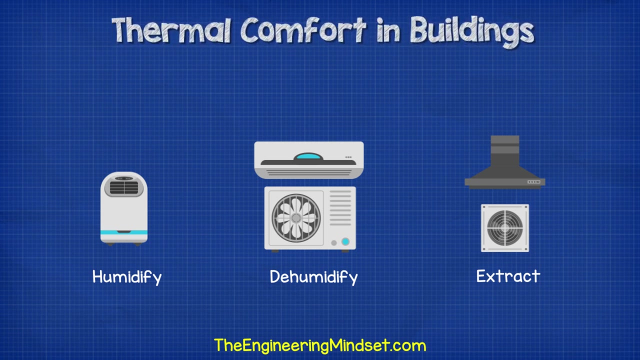 very comfortable and quite happy sitting here in a t-shirt. Things like kettles or water boiling showers or even drying clothes will all add moisture to our environment, so we want to try and isolate these and keep them separated and well ventilated. In homes, we can control the humidity using small portable devices, but 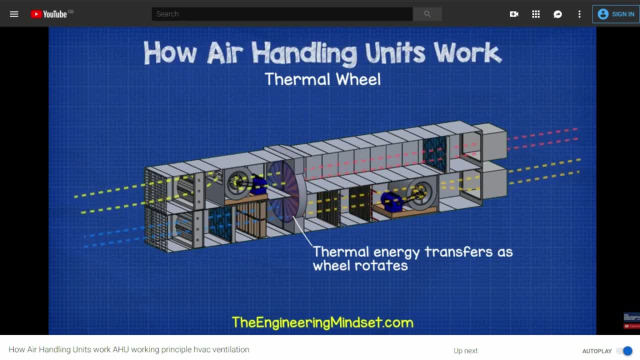 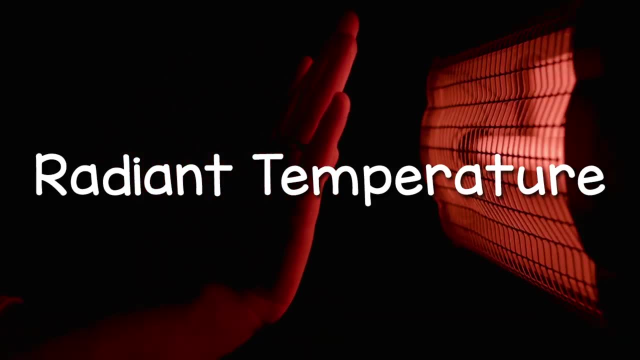 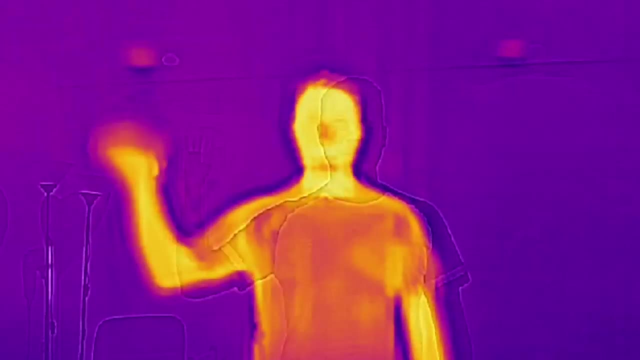 in large office buildings we tend to use the central ventilation systems. Again, we've covered that in another very detailed tutorial. Radiant temperature: This is the temperature of the surfaces which surround the person. It's thermal radiation. Everything, including you, give off some thermal radiation due to 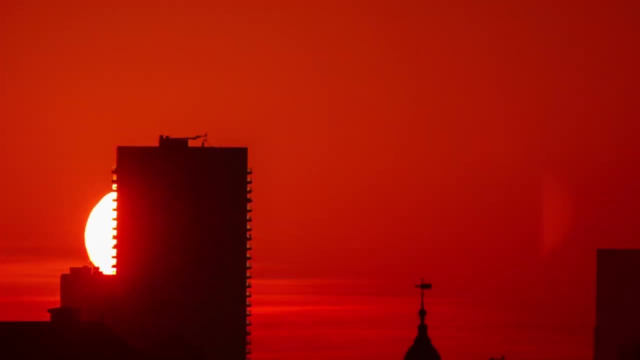 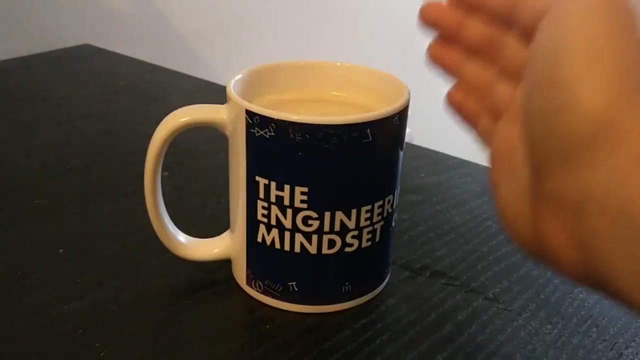 the differences in temperature. We can feel this when the sun shines on us or even just reflects onto us. We can also feel it when we walk past a hot oven or some heated material, And we can even feel it when we place our hand in proximity to a hot cup. We can visually 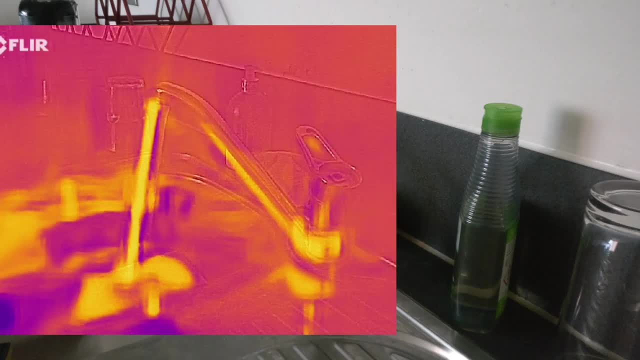 see the source of the heat using thermal radiation. We can also feel it when we walk past a hot oven or some heated material, And we can even feel it when we place our hand in proximity to a hot cup. We can also feel it when we place our hand in proximity to a hot cup. 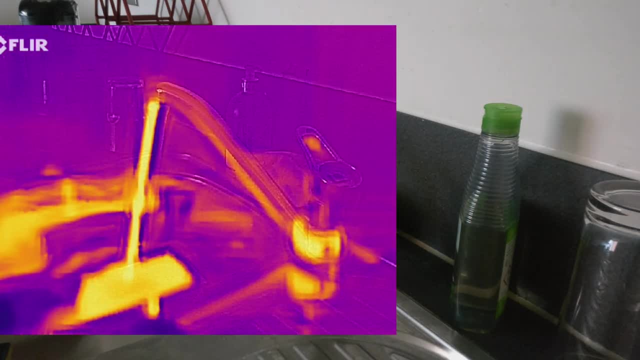 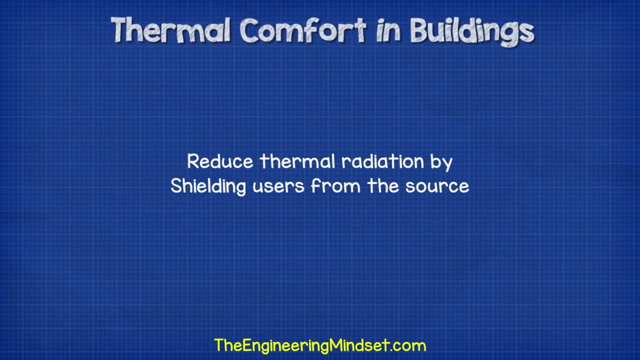 Now, these shots I filmed using a pocket sized camera which attaches to my smartphone, and I use it for inspection and troubleshooting. I'll leave a link down below if you want to check that out. We can improve or reduce the radiant temperature by basically putting a barrier between us. 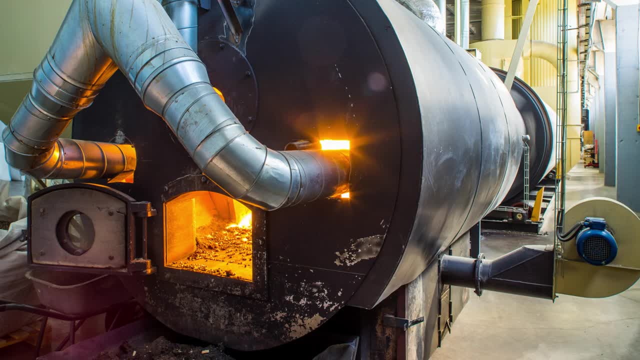 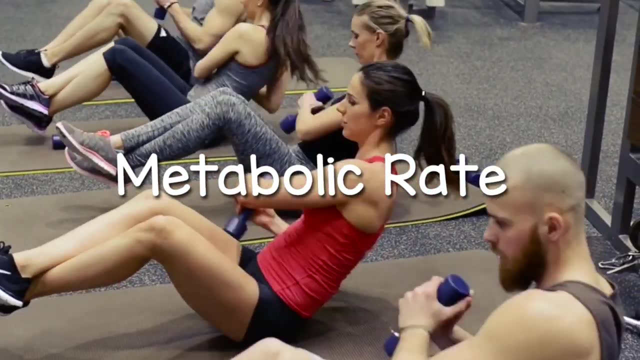 and the heat source. Whether it's a shade, a wall or insulation, we just need to block the path of the thermal radiation Metabolic rate. This is how much energy our bodies will burn, and it's mostly associated with a person's level of activity.